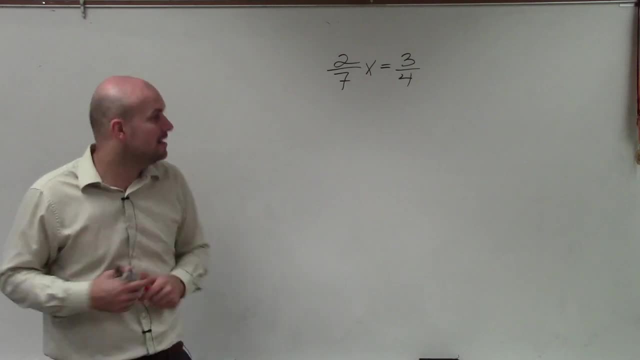 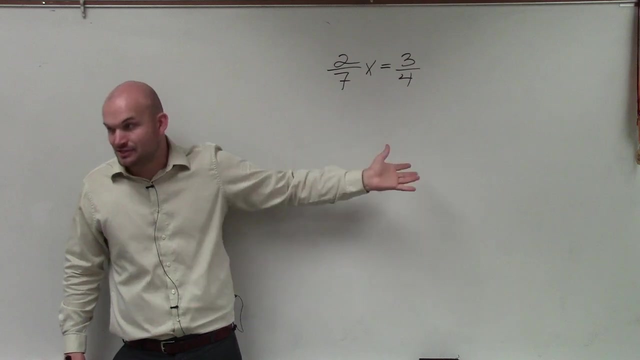 with it now, because that's what we did in the last test. But when you get into more complicated problems, I think it's always easier if you can just eliminate the fractions. It makes life a lot easier. So it's important for you guys to understand. why do we have 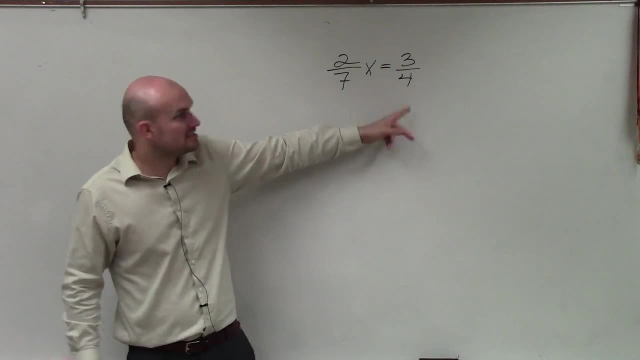 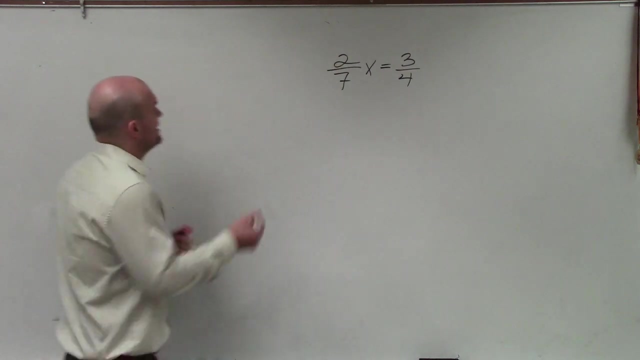 fractions. We have fractions because 4 does not divide into 3.. Does that make sense? We have this fraction because 7 does not evenly divide into 2.. We can get rid of a fraction if we have a denominator that easily divides into the numerator. 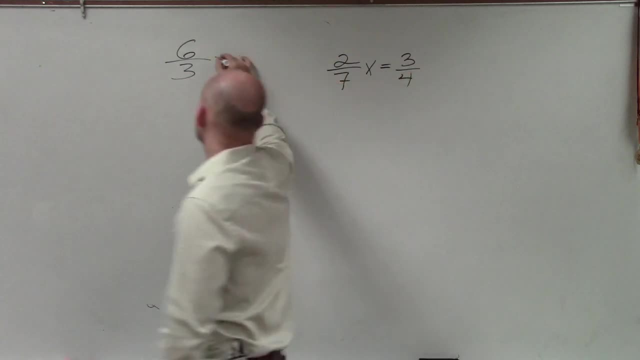 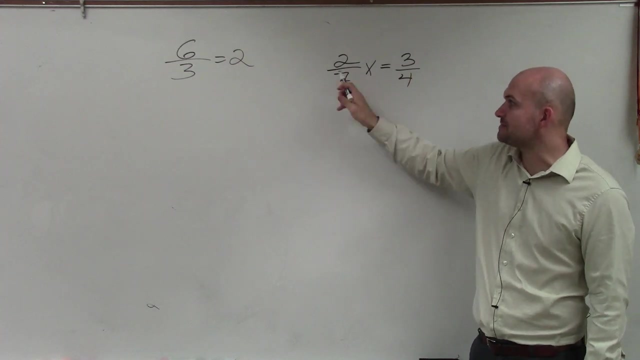 Right, We don't have to keep this as a fraction: 6 divided by 3, we can just reduce as the whole number, 2.. So when you have fractions, you need to understand why we have fractions. We have fractions because the denominator does not divide into the numerator. So to 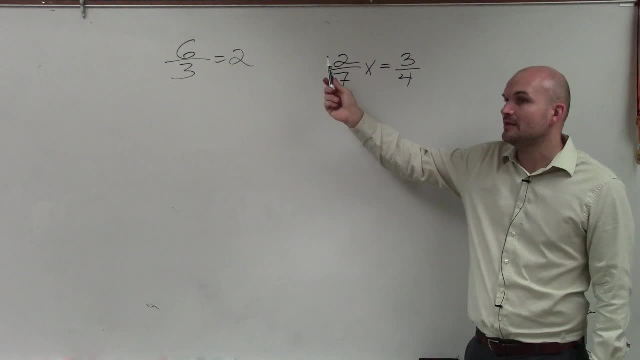 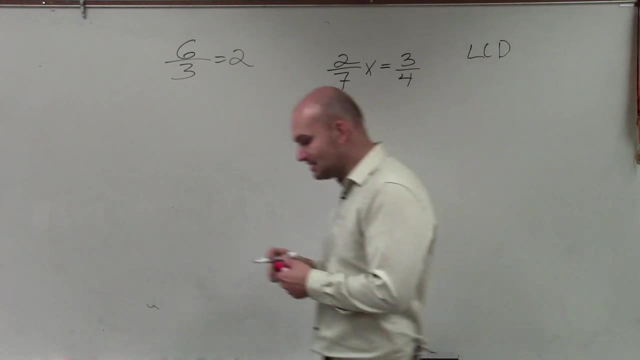 get rid of fractions. we just need to figure out what number that we can divide, both a 7 and a 4.. So we need to determine what we call the L, C, D. What is the least common denominator, the smallest number that both 7 and 4 divide into? 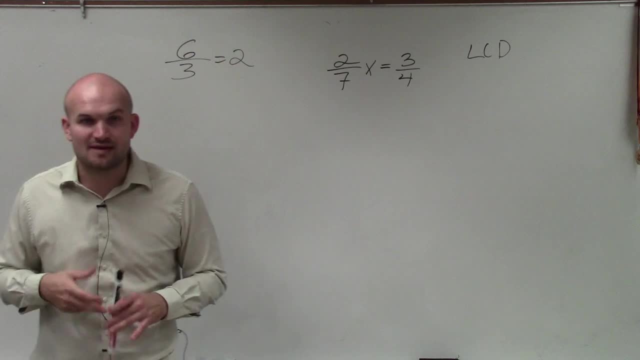 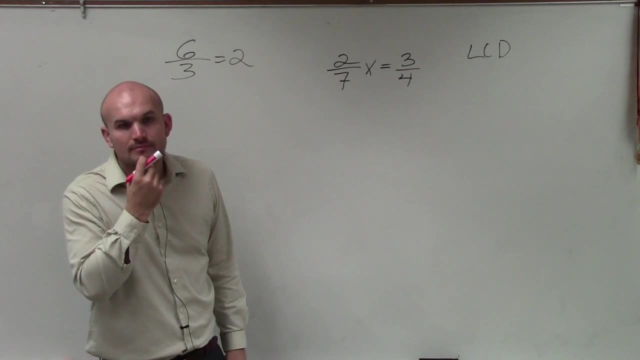 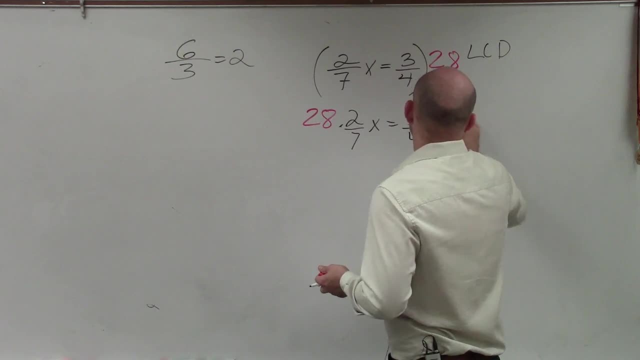 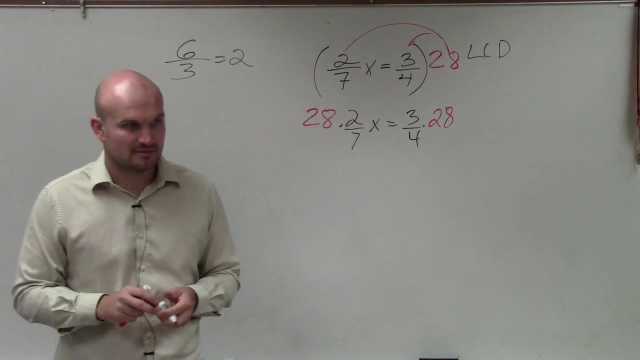 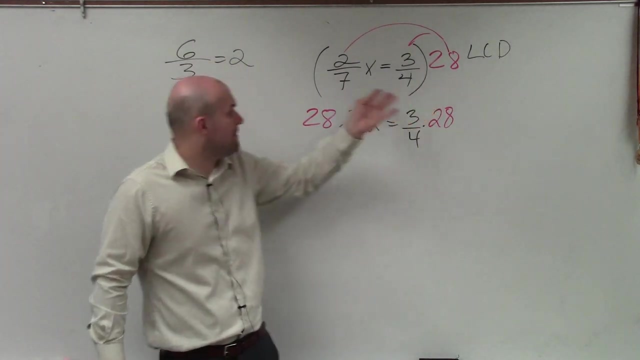 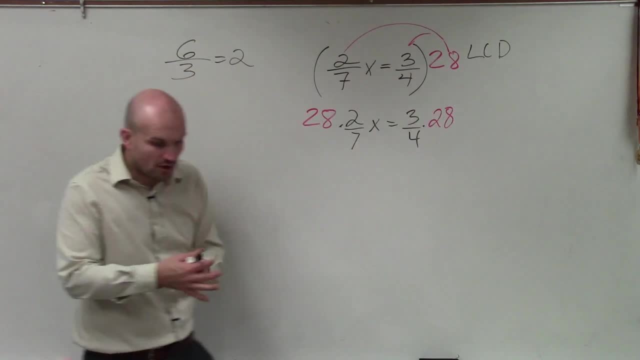 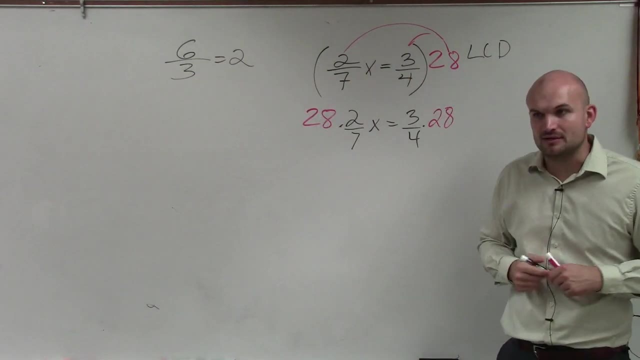 and 4 divide into correct Yes, So guess what? We chose a number that now our denominators divide into. How many times does 7 divide into 28? 4 times. So I can simplify that fraction and just write 4.. 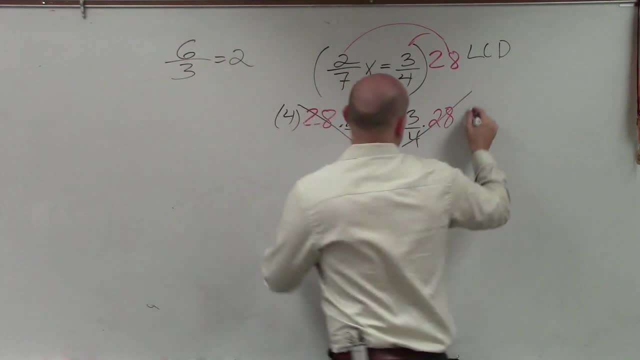 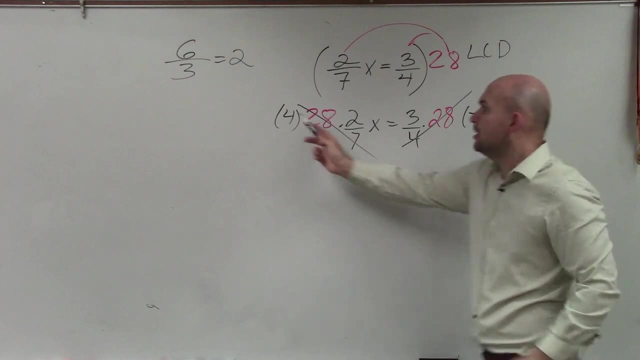 How many times does 4 go into 28?? 7. So now I eliminated the fractions because I divided them into the number. 4 times 2 is 8x. 7 times 3 is 21.. Divide by 8.. 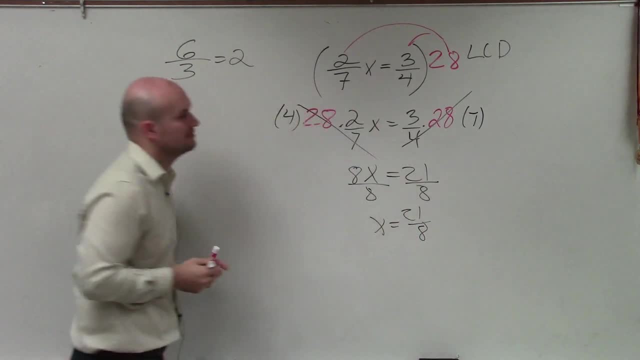 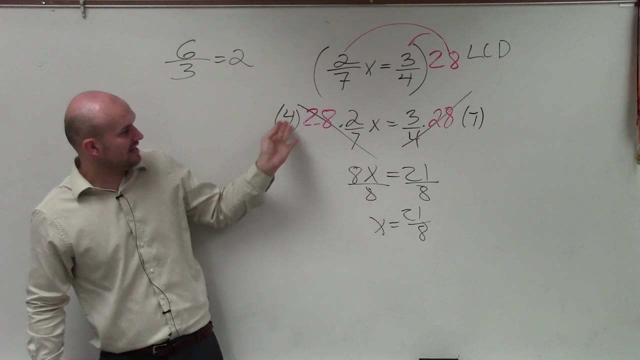 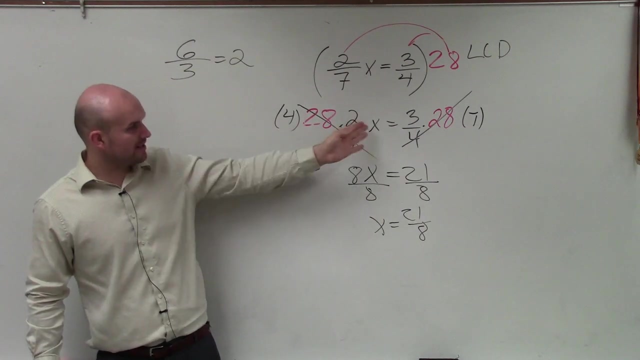 Divide by 8.. x equals 21 eighths. Do you understand how I went from 7 to 28,. gave me 4? Then you just multiply it across 4 times 2.. 8. 2 is 8.. 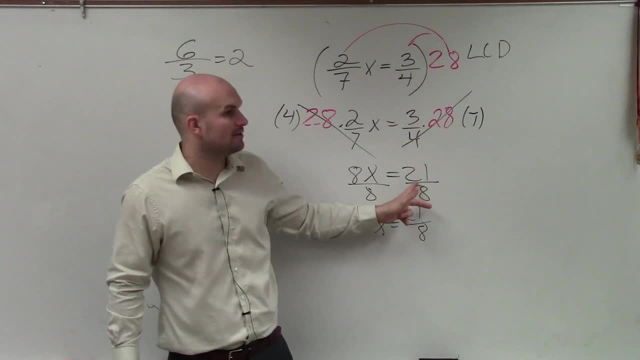 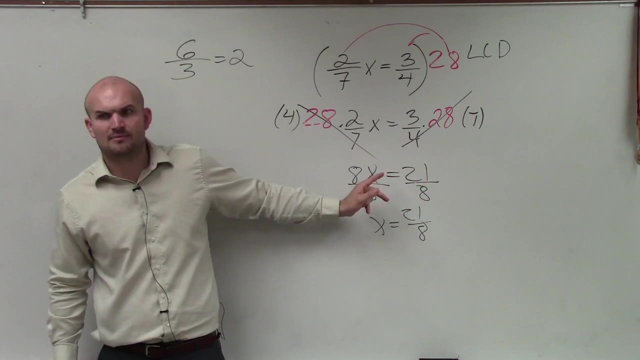 4 divides into 28, seven times 3 times 7 is 21.. Then I have 8x equals 21.. Excuse me, Excuse me, I don't know why I'm competing with anybody else. So do you understand how I at least got to this part? 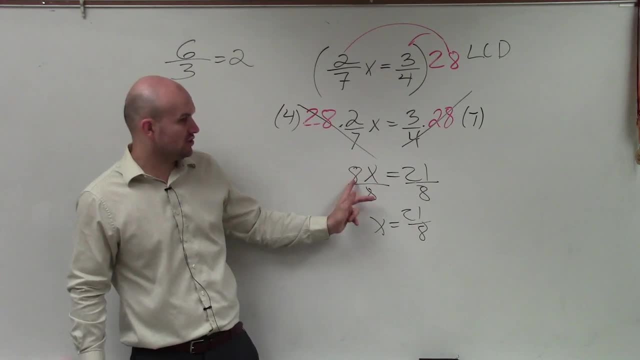 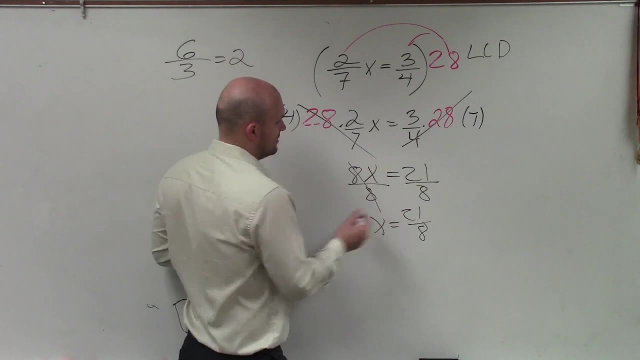 OK, Now my variable is being multiplied by 8. So to undo the multiplication, I divide by 8 on both sides. That divides out to 1. And I'm left with 8.. x equals 21 over 8.. Jamie, yes, 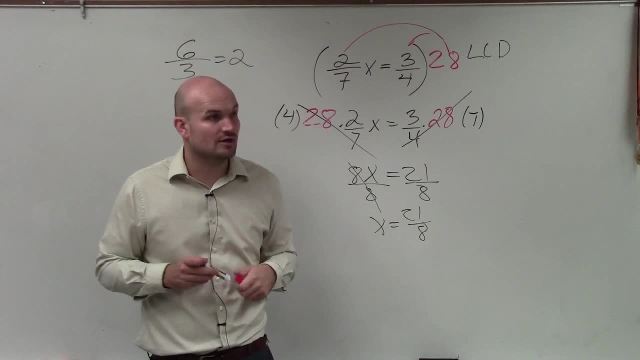 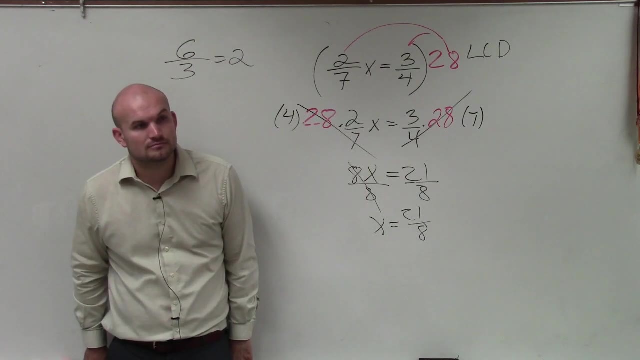 Amy, yes, No, Sit down, sit down. Let me go over this. You guys are wasting your time. Is there any easier or different method that we could use for solving this particular equation? Absolutely. Do you want me to go over that with you? 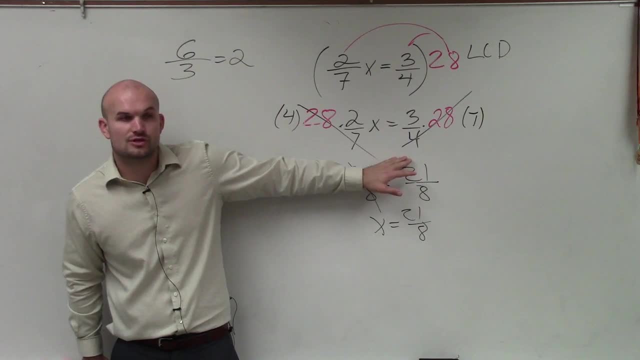 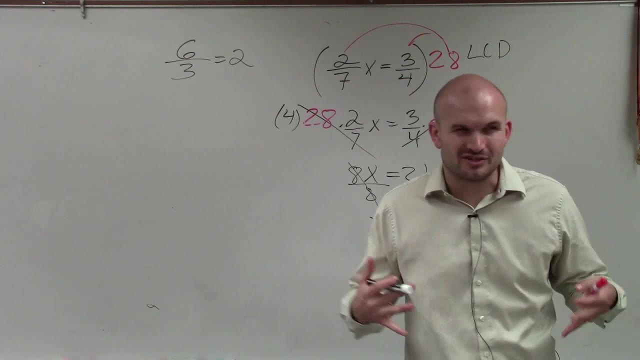 Because I showed you guys the first way, I'll give you a second. The reason why I showed this way, Austin, is because when you guys are working through problems, as I mentioned, This isn't as important in this one. But if you guys don't know how to eliminate fractions, 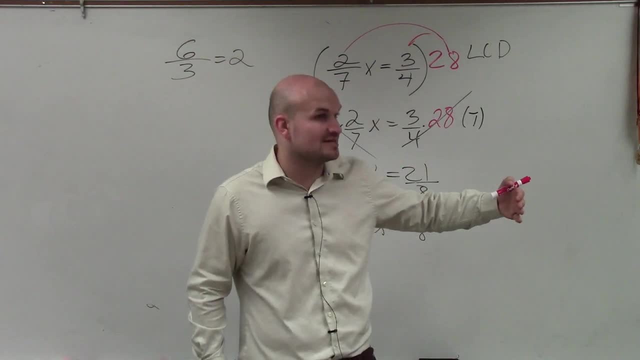 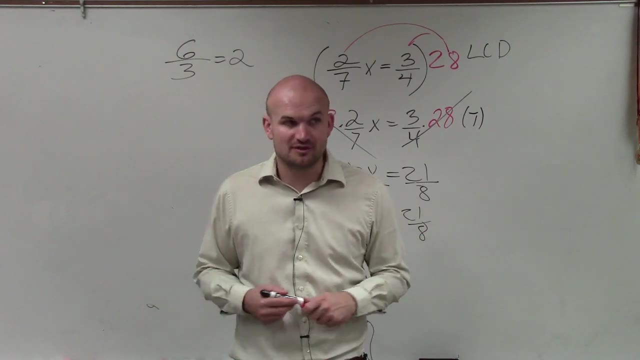 I think it will be very difficult to start doing harder problems, that we're going to go through with fractions, Because then you're going to be adding, subtracting, You're going to have to find common denominators. It can be sometimes difficult. 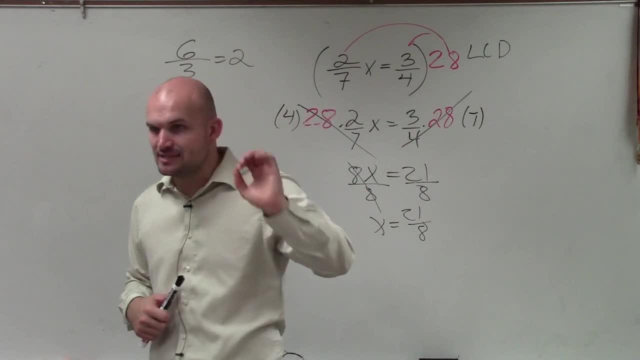 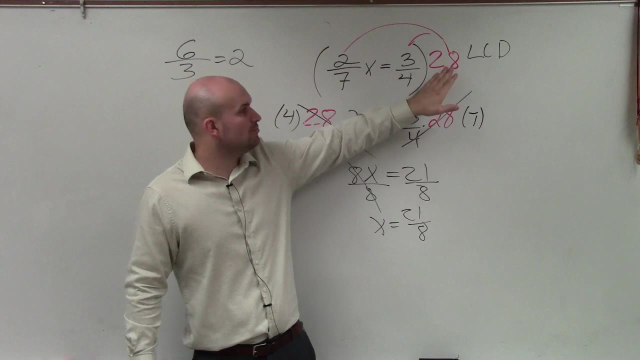 So when you have fractions, one method to always apply is to get rid of the fractions. How do you get rid of the fractions? Multiply by the LCD. When you multiply by the LCD, your denominator, your denominators, now divide into that LCD number. 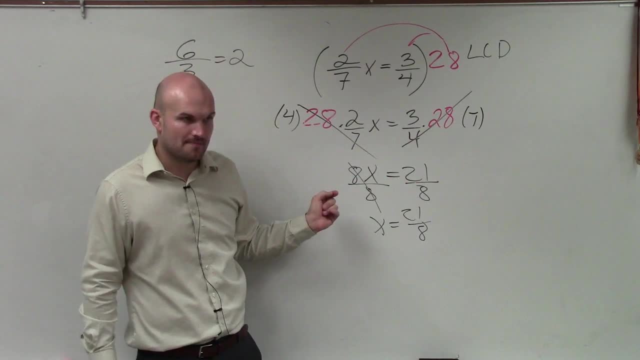 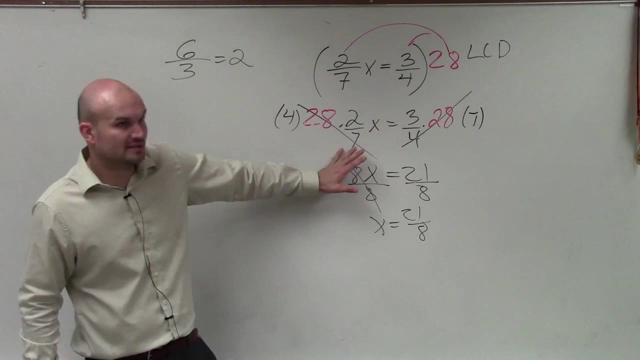 And you can simplify it without fractions. So this is a longer way to do this problem. However, once we get into multi-step and two-step, this is going to be probably a preferred method. Now let's go over the second way to do it.